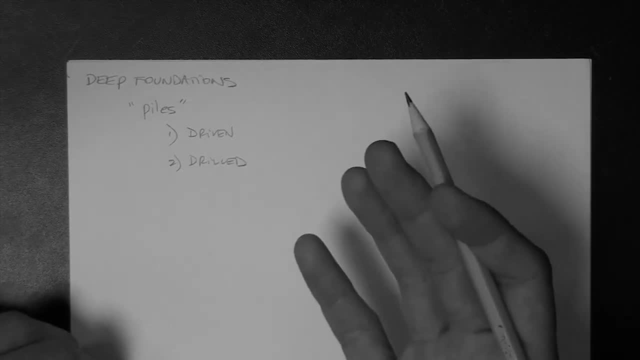 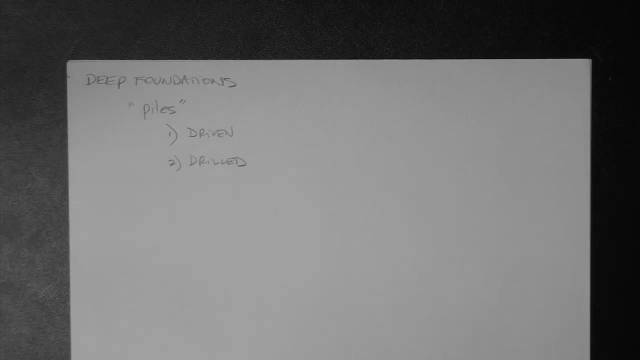 piles that are used interchangeably. Now there are different names for, for example, for drilled some people use. instead of saying drilled piles, they would say something like drilled shafts or something like drilled caisson, something like that. okay, but in general, if you speak of driven piles and drilled piles, I would say all. 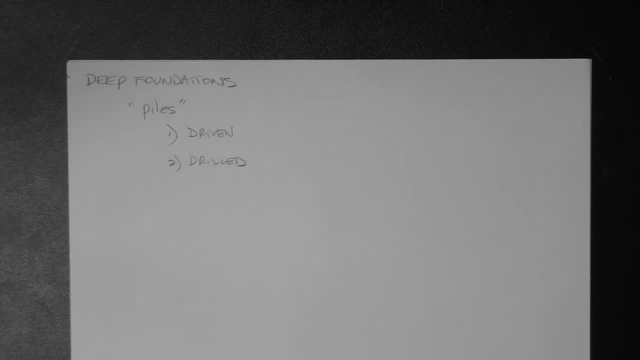 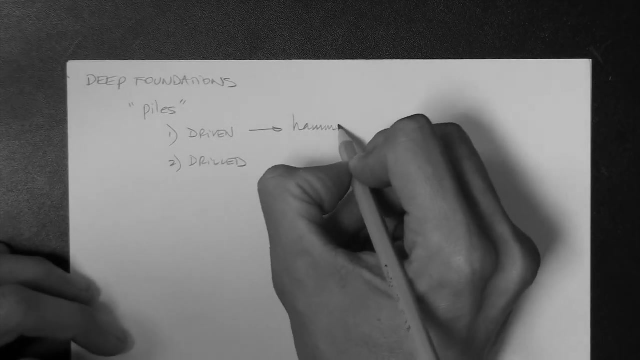 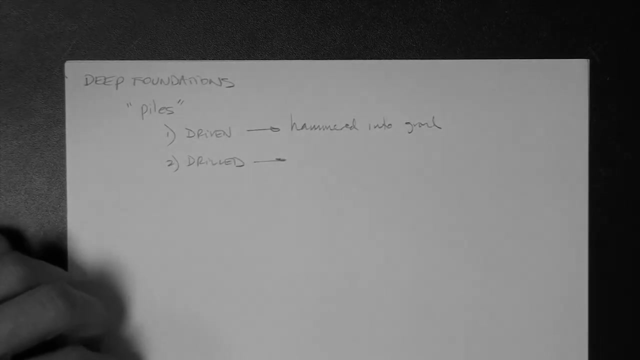 your technical engineers that know what they're doing will will understand you. okay now, driven piles are essentially driven into the ground. okay, they are piles that are driven or hammered, let's say into the ground. so we're going to use that word: hammered into the ground. drilled piles are constructed, let's say underground, okay, so we'll just write. 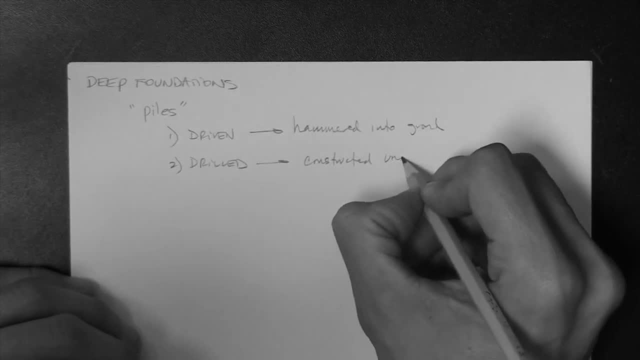 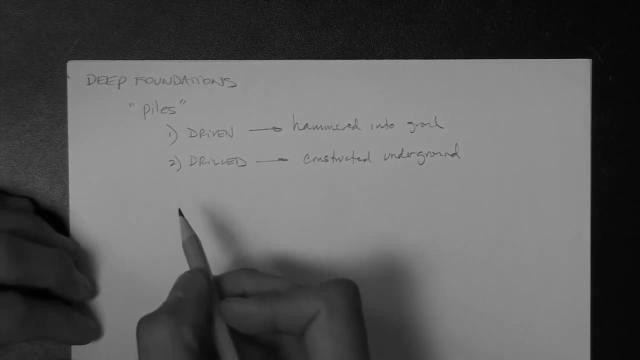 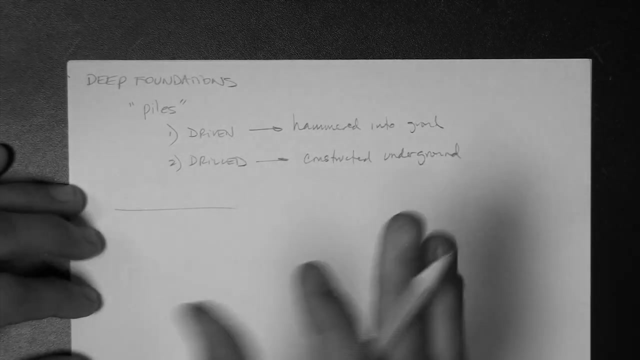 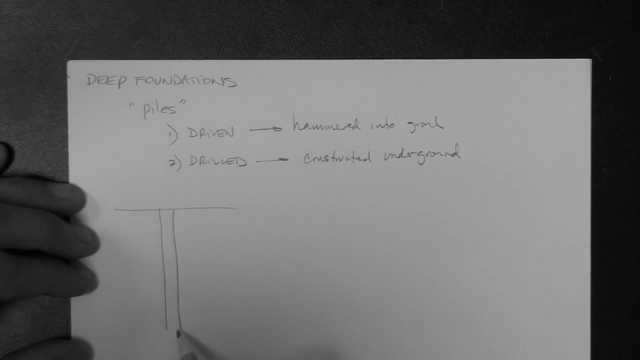 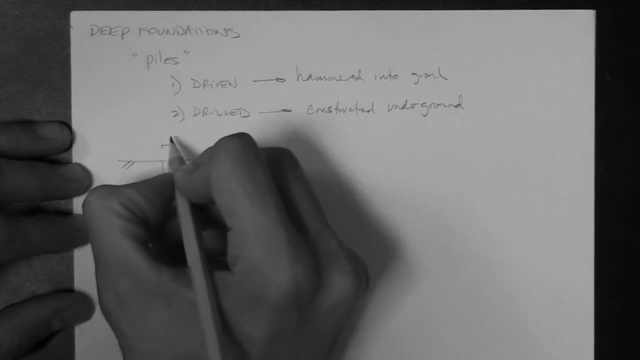 that constructed underground. all right, so well, let's go out. let's actually describe what a pile looks like. generally, a pile looks like this. this is regardless of whether it is driven or drilled. okay, it essentially looks like a submerged column. okay, so this is a ground surface and this is the width or diameter of the pile, which, as you know, 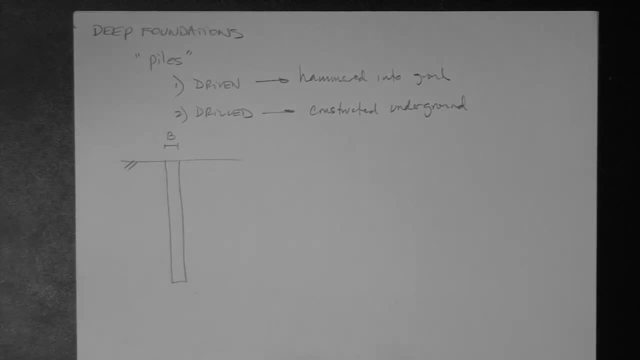 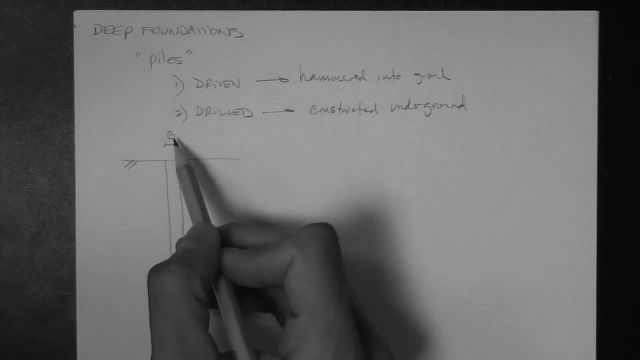 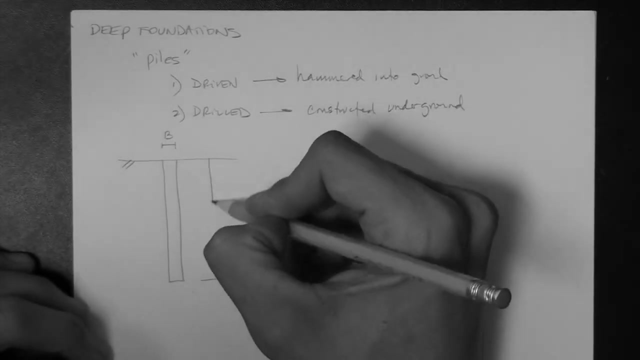 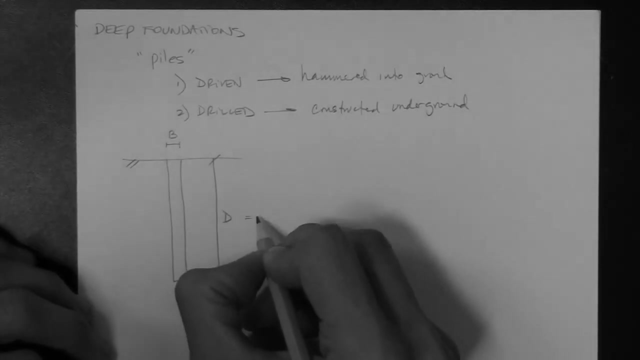 from your foundation studies. generally, the width of a footing or of a mat or of a pile is termed, or the letter b is used to term the width. okay, so the letter B, capital B. okay, a pile has a length d, which is the embedment length, right? 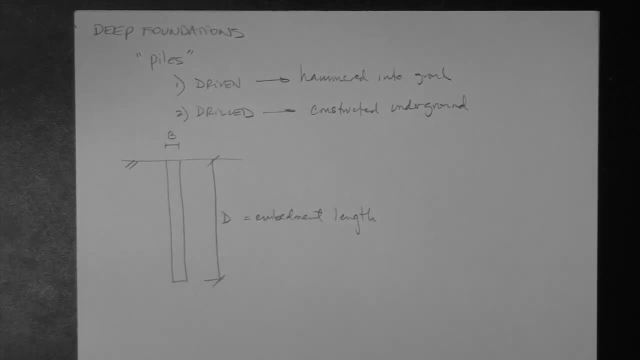 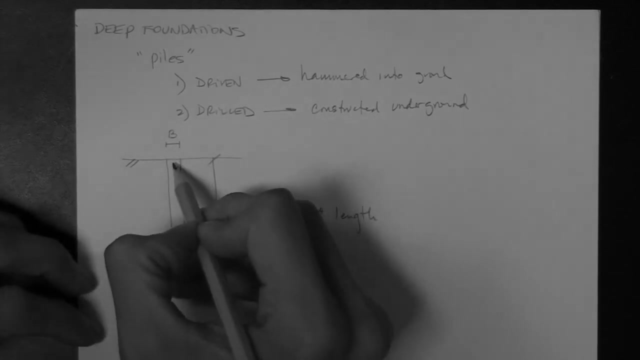 okay, and essentially that's what it looks like. generally a pile is made of a- I would say I would say most piles. I would just say this, even though I don't really know the statistics, but I would say I would guess that most piles are circular in cross-section. so this right here. if you were to look at from the top. 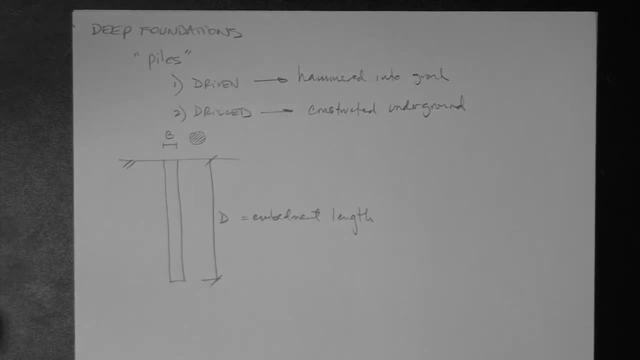 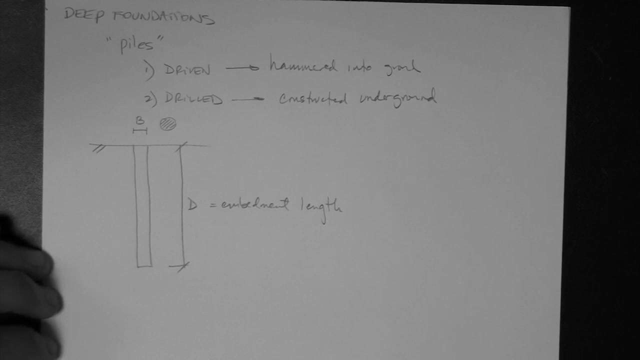 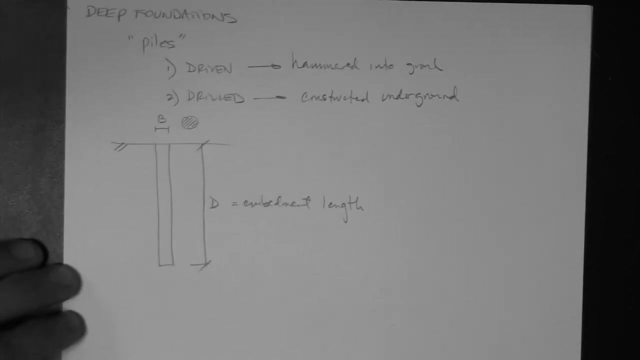 it would be something like that: okay, and the diameter is B, but you could have piles that are, that have different cross-sectional shapes. it could be a square pile, or even maybe an octagonal pile, etc. okay, all right, let's go back to the driven versus drilled, so I'm going to just move this up. well, clearly, the 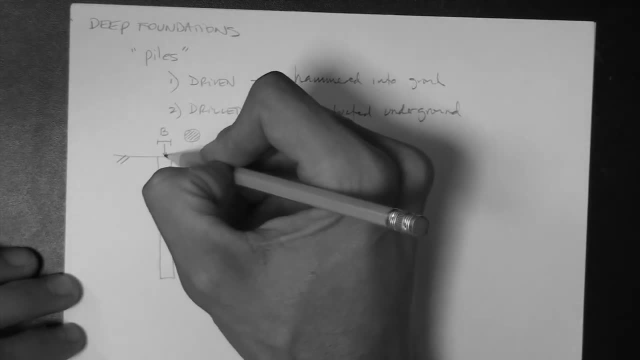 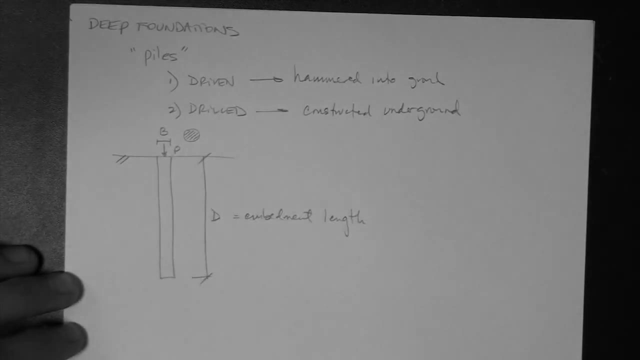 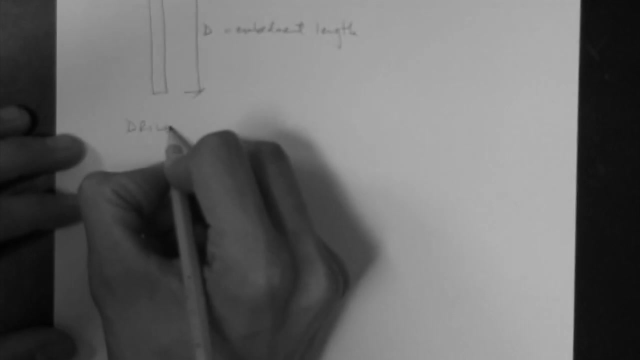 load. the axial load on the pile is applied as denoted by that arrow right. this is the column load, for example, column axial load B. all right, well, let's go back to the drilled versus driven. so a driven pile. this is remember. this is very quick. there's a lot of stuff to 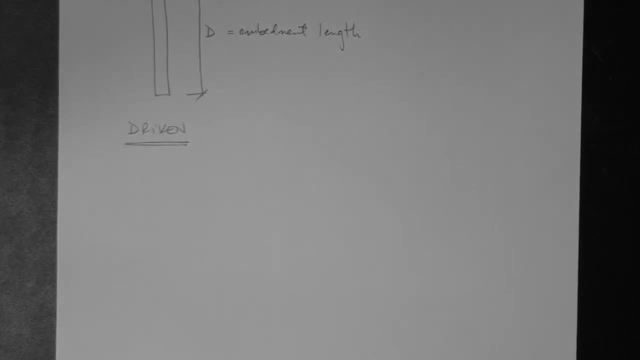 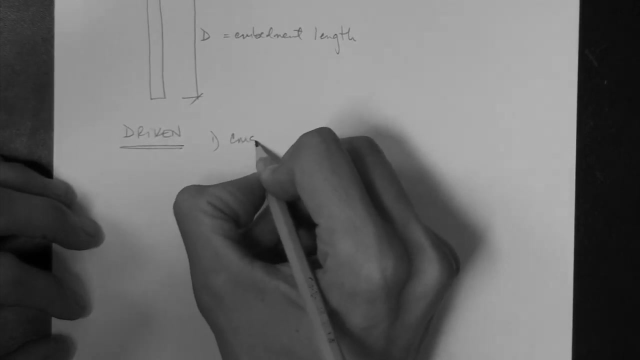 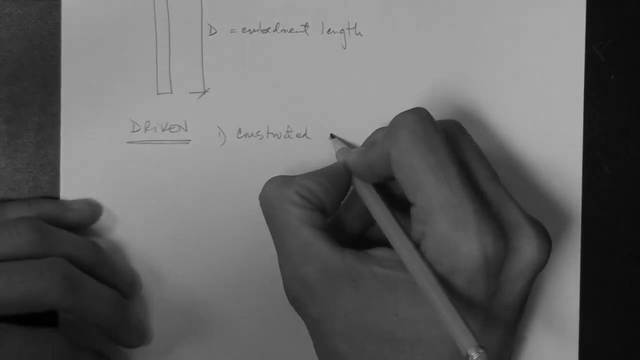 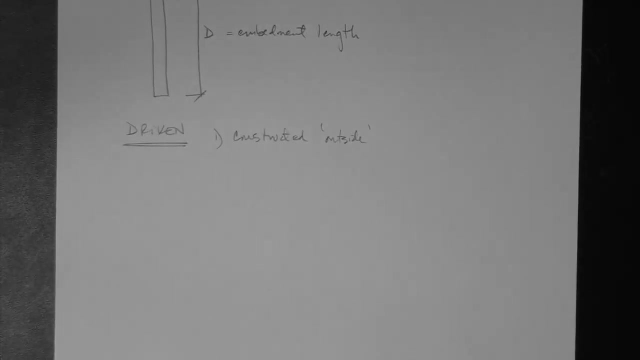 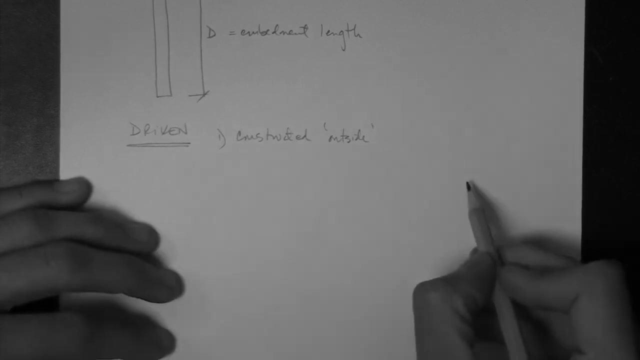 read about this, the types of piles, etc. and this is very general, but I think it's the fundamental stuff. okay, so a driven pile is constructed outside of the ground? okay, outside, let's say okay. so basically you could take, for example, a light post. imagine a concrete light post, the ones that are used, let's say, if you have like. 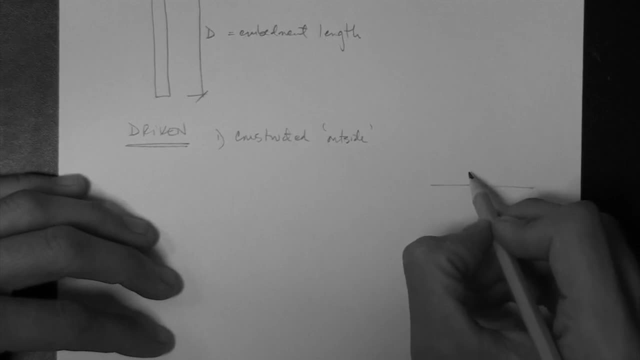 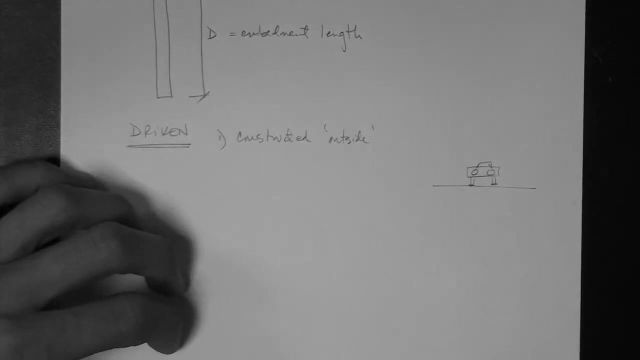 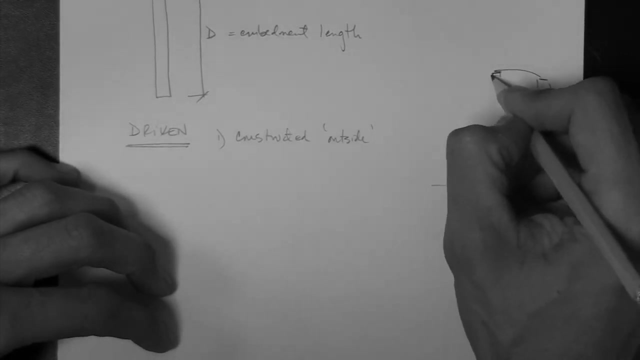 a you know, a roadway. the cars are going into the right. sorry, but let's say these are the lights, so the car is coming out of the page like this. okay, so we have light posts, which are basically columns with a light on top right to to provide light to the 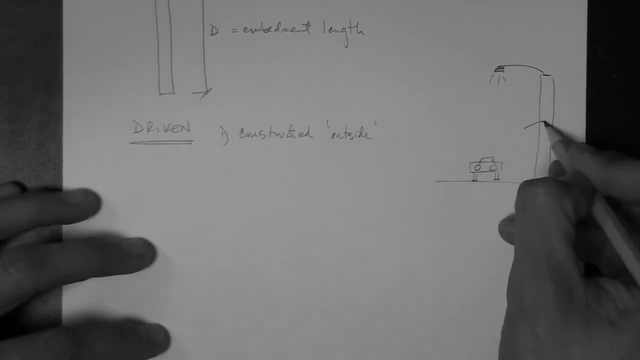 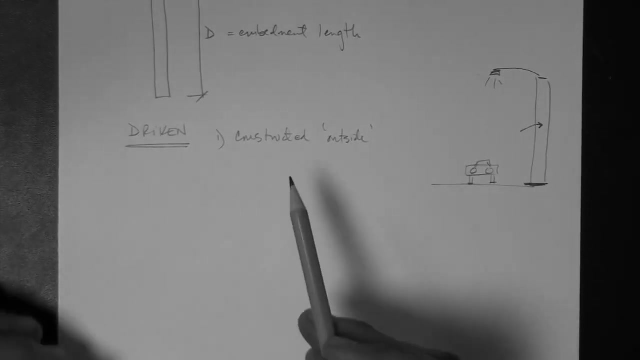 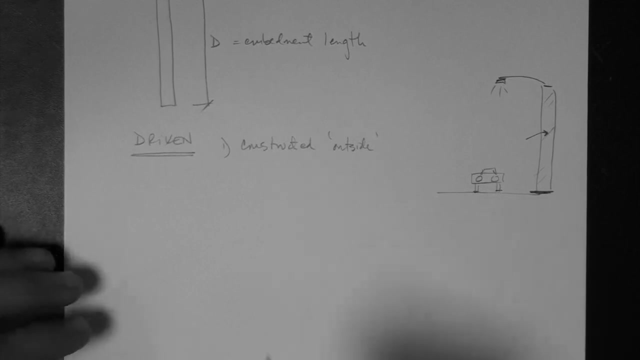 to the, to the street. okay, if you take this light post and you hammer it into the ground, you create a driven pile, okay, so what I'm trying to say here is that you can take something that is already constructed, or you can construct it on purpose, to then drive it or hammer it into the ground to create a 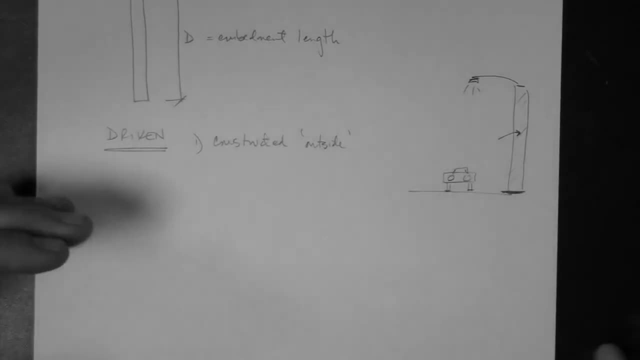 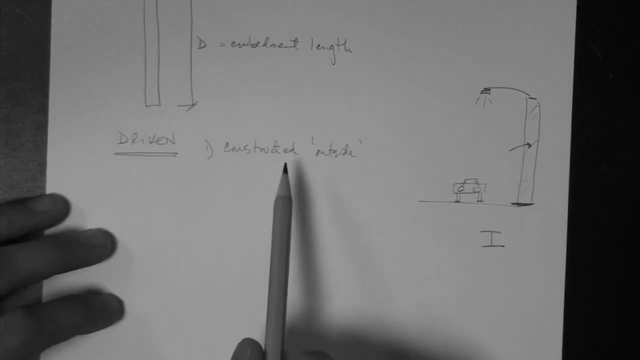 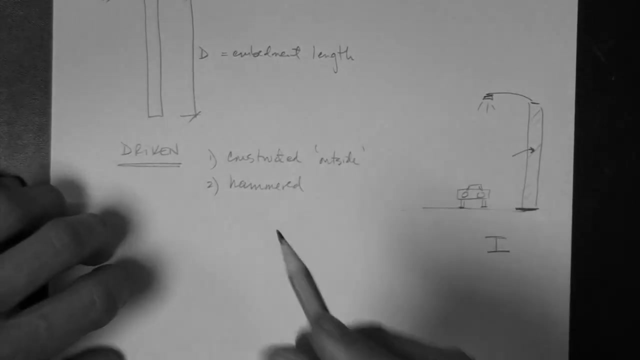 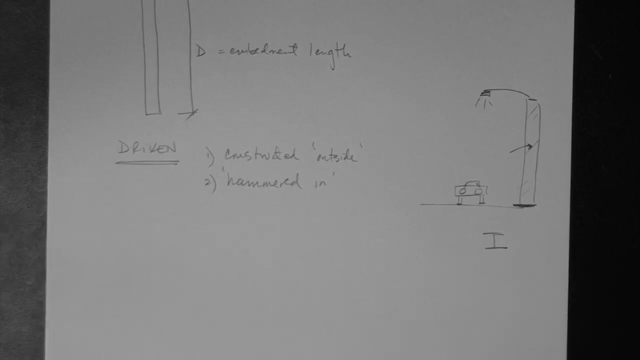 pile. ok, you could take a steel pipe, for example, and do the same, or an I section- okay. anyway, these are constructed outside of the ground and then hammered in. I already wrote this, but, okay, hammered in. so what does that mean? well, there are typically very large equipment that are taken to the site and this equipment holds. 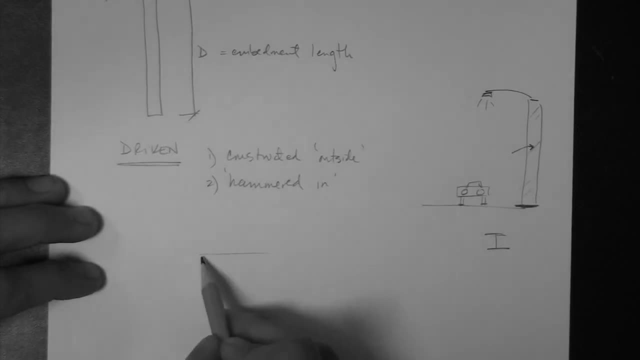 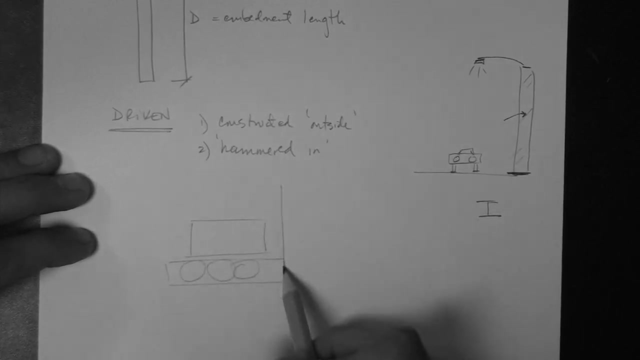 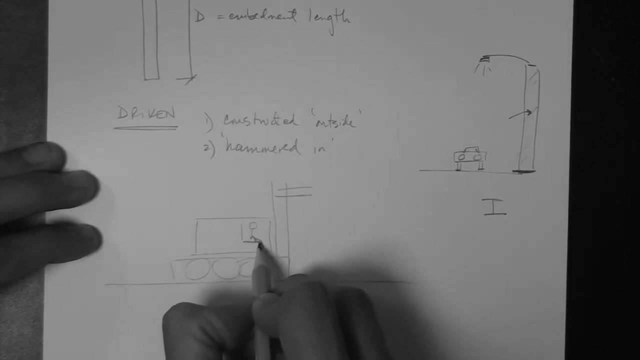 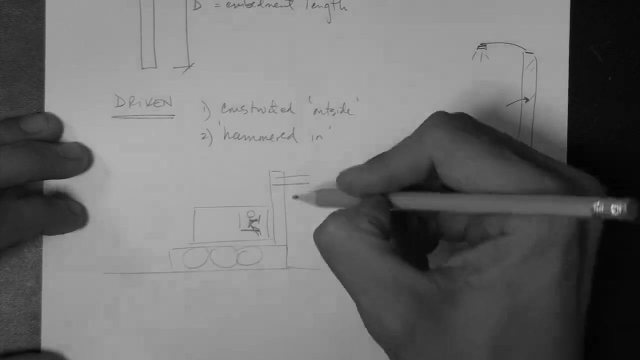 the pile vertical. okay, so the equipment may look almost like you know one of those heavy construction equipment etc. it has a holder. this is the ground surface. there's a person here- maybe you know driving this thing. okay, sorry for the little mess, but there's a holder here that places the pile. 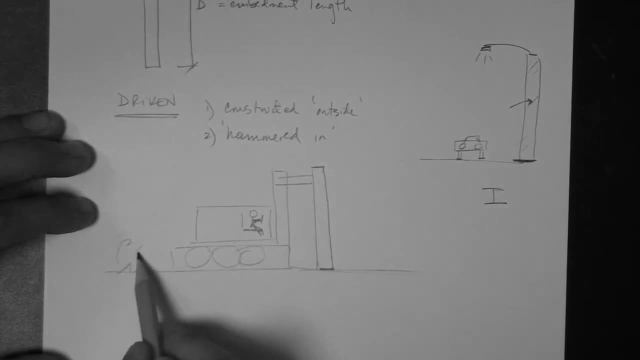 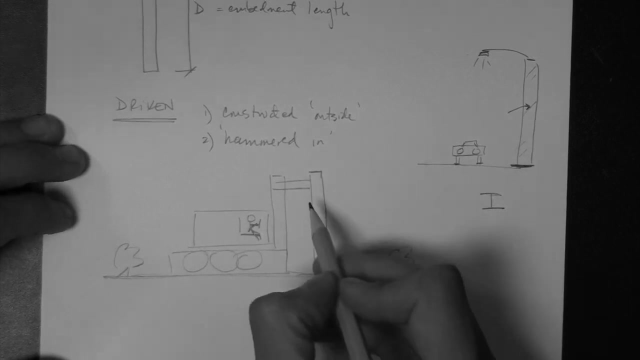 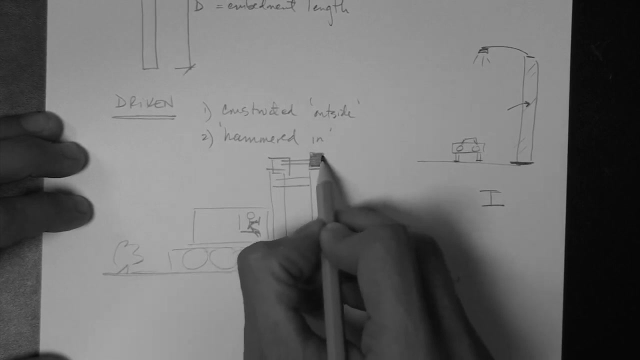 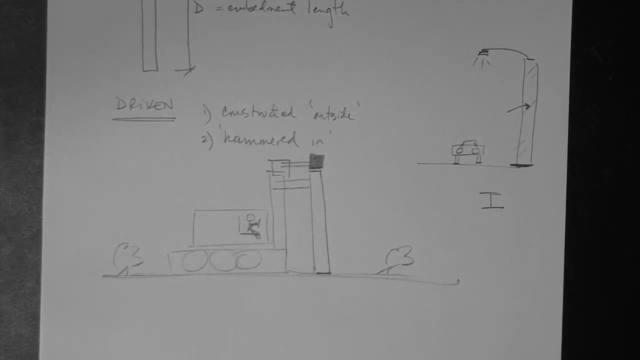 on the spot. these are trees, okay, let's say around surface right where it's going to be driven, and then in here. this is very rough, but if you go on YouTube you could just type in driven pile installation or something like that and you will see obviously very nice videos on how this is done. but essentially this: 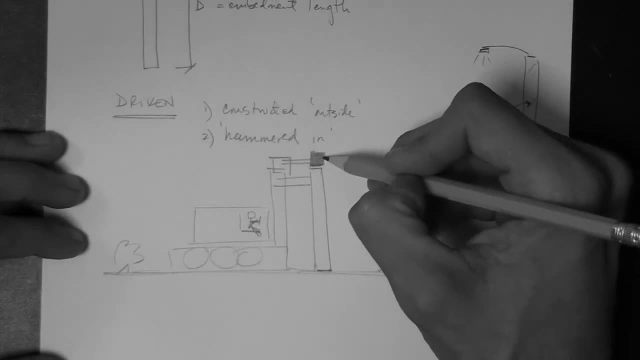 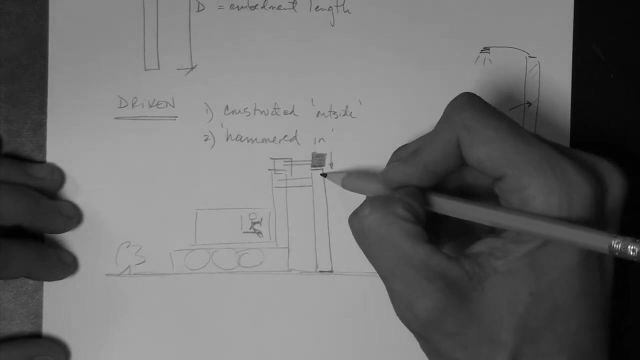 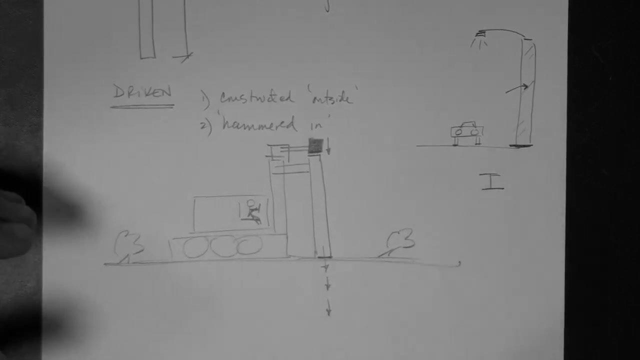 machine holds the pile vertical and then this hammer is raised and then released so that it actually hits the top of the pile and the pile is literally hammered into the ground, just like a nail would if you hammer it with a wood hammer. you know a wood nail if. 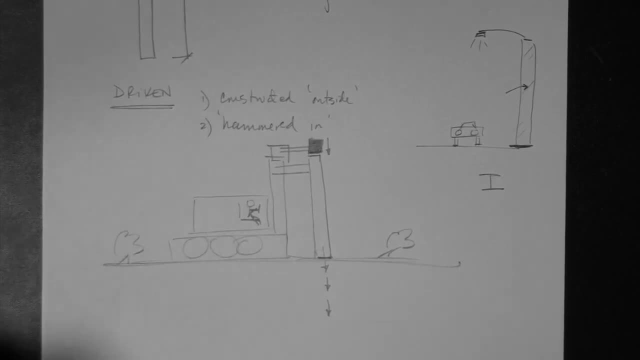 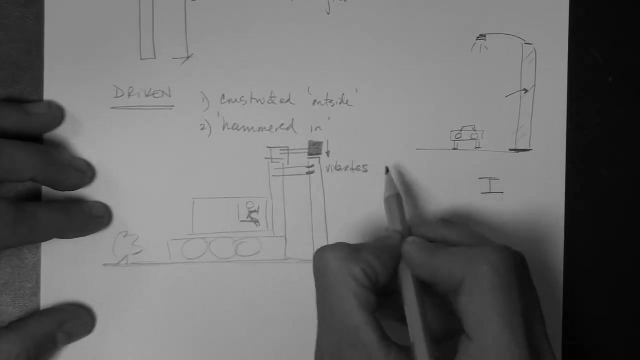 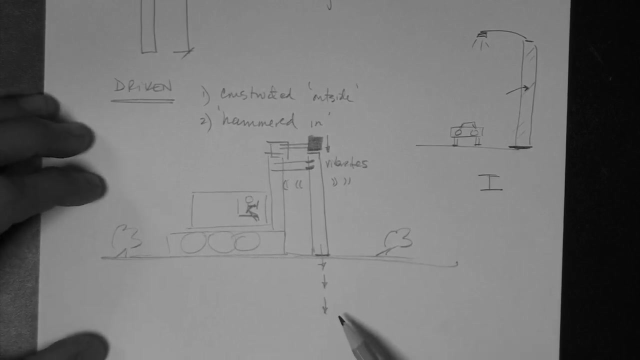 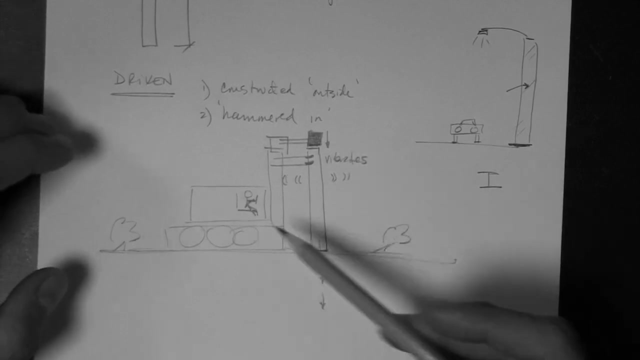 you hammer it in to a piece of wood, for example. same thing, same concept. in some cases- I would say most cases- this part here vibrates, so there's vibration incurred. okay, and generally when you have coarse grain soils, even fine grain soils, if you vibrate the pile while you're hitting it, then it's most of the. 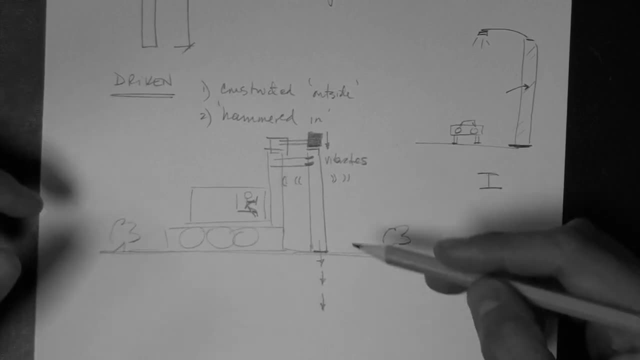 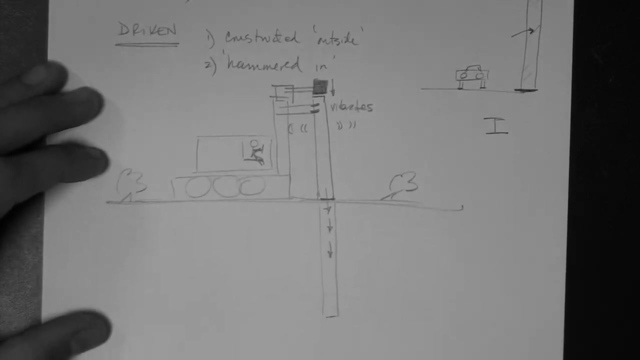 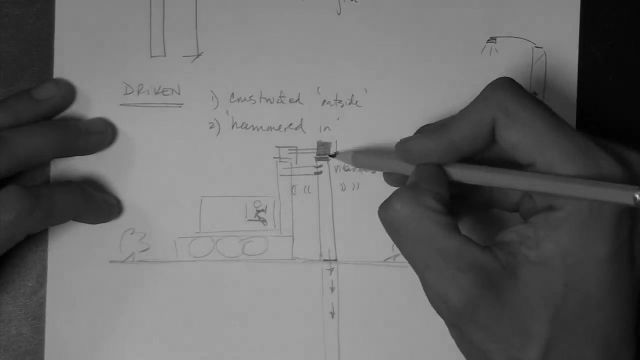 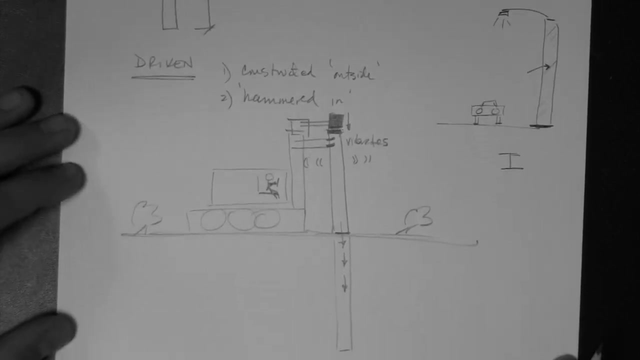 machine is more effective in being able to drive the pile or place the pile into the ground right, so the pile comes in and in and in, and then eventually it's down here. okay, there is generally a cushion that is placed at the top so that hammer does not break the top of the pile when it's hitting it. okay, so driven. 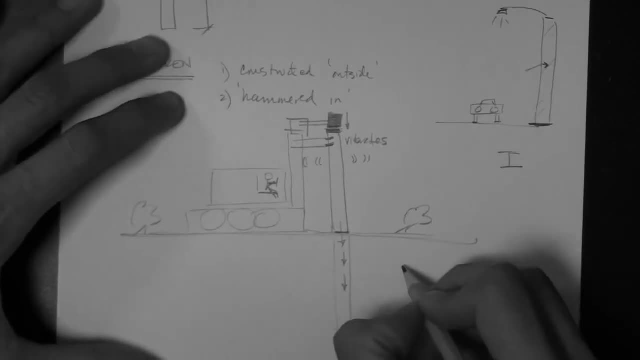 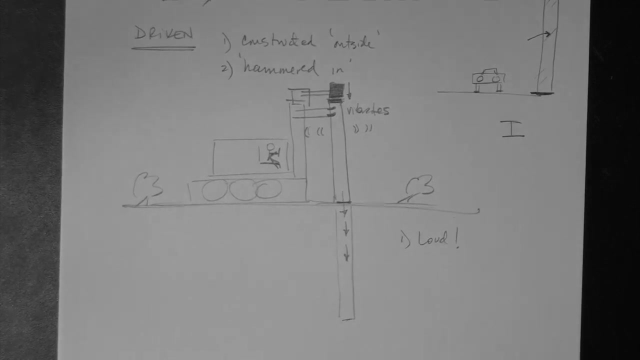 piles are essentially constructed this way. all right, now a few things. one: this stuff is loud, okay. so if you have a project where you're going to construct a building, let's say next to a hospital, okay, or something like that, generally you would prefer perhaps not to use driven piles, because then 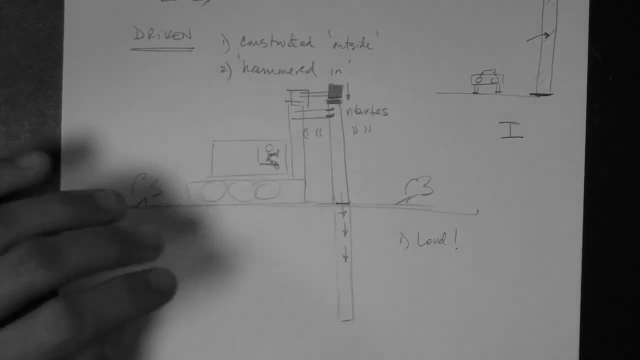 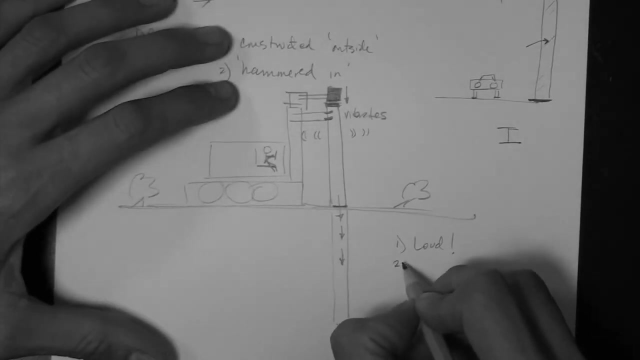 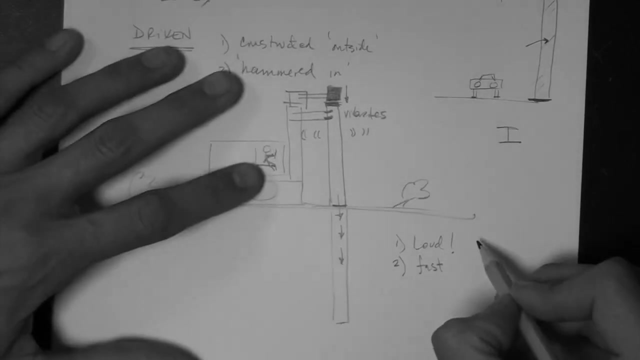 it would create a lot of noise, etc. right, so these are. this is one of the kind of disadvantages of, lets say, driven piles. number two: generally this is a fast installation, so this is kind of like an disadvantage. this one is an advantage because remember that fast construction. 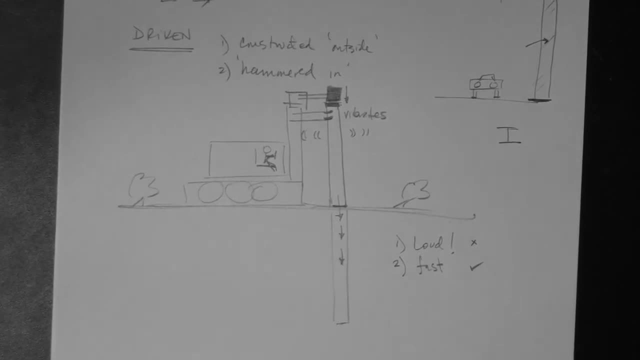 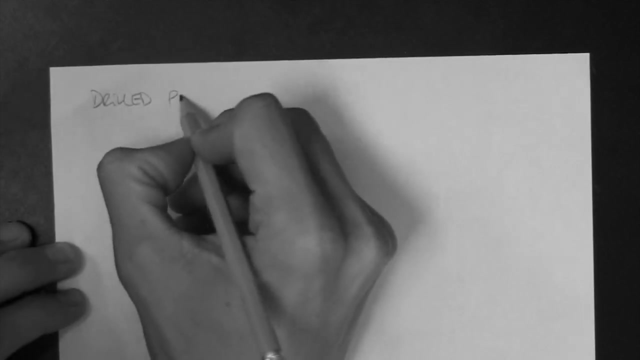 means that it's a fast construction. that is not going to happen right now. So that's one of the important things that I want to emphasize. means generally means that we're making more money than if we construct slowly. Alright, let's talk now about drilled piles. 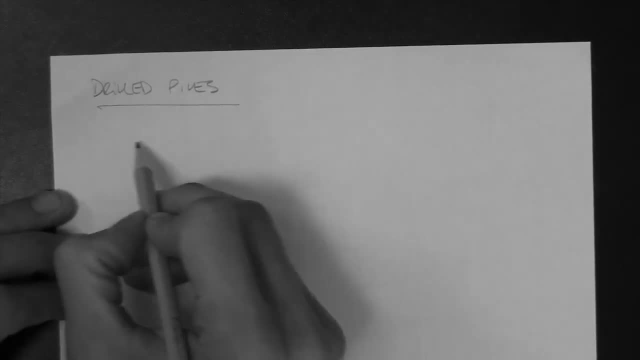 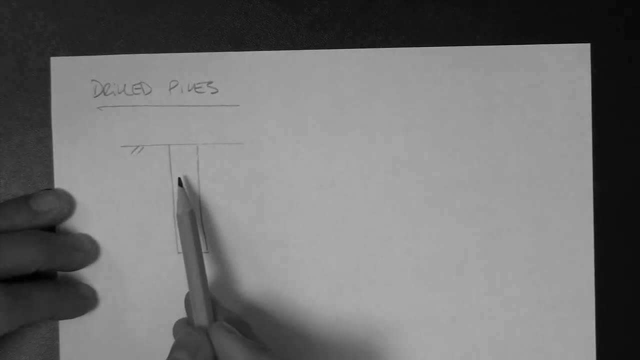 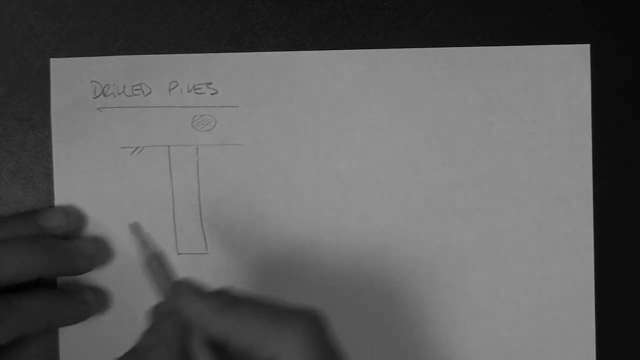 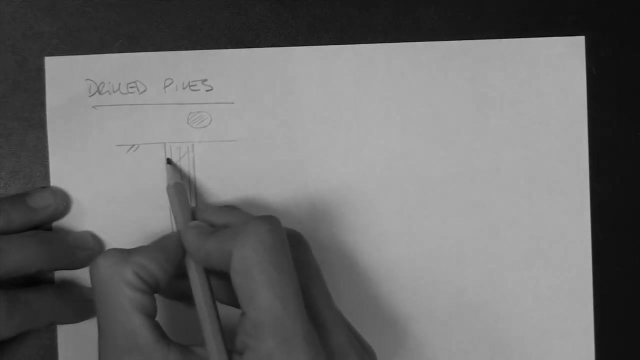 Drilled piles are piles that are essentially constructed in the ground. So, essentially, what you want to end up with is a essentially a concrete column, generally circular, again in cross-section. okay, that is basically submerged in the ground, Reinforced concrete, which means that it has a rebar cage. 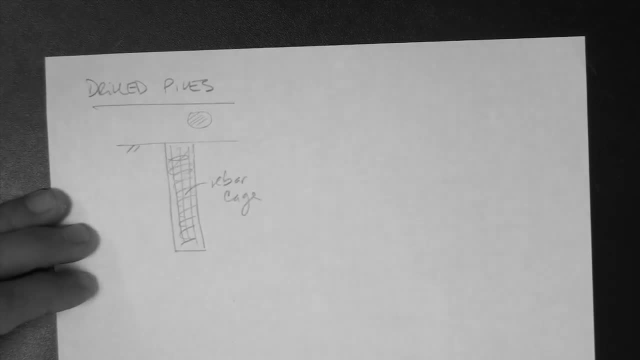 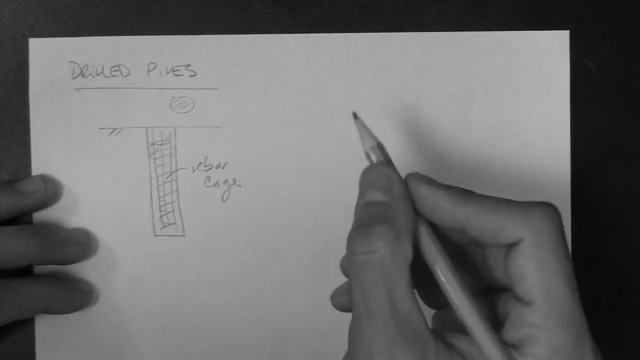 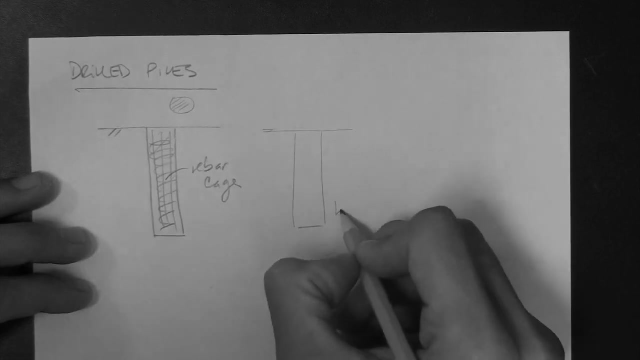 Okay. now there are various ways in which this can be achieved. So there are piles that are, for example, constructed as follows: You dig a hole, Okay, And the hole is dug with what's called an auger, which is essentially a large drill. 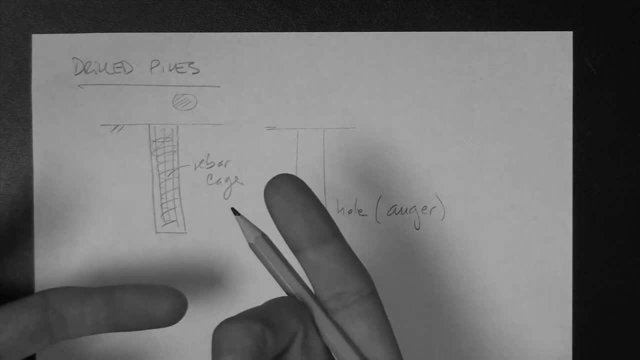 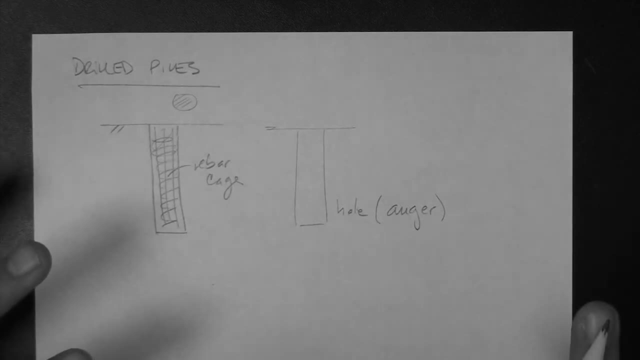 bit, as in the drill bit that you would have in a hand drill- okay, but it looks a little bit different. It's wider, with flatter wings, okay- than a hand drill drill bit. So what I'm going to do is I'm going to upload some videos or I'm going to provide some 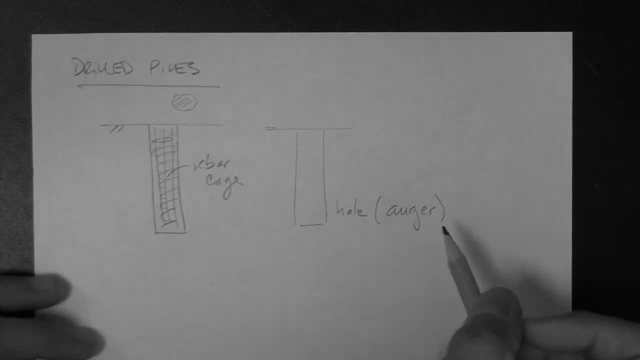 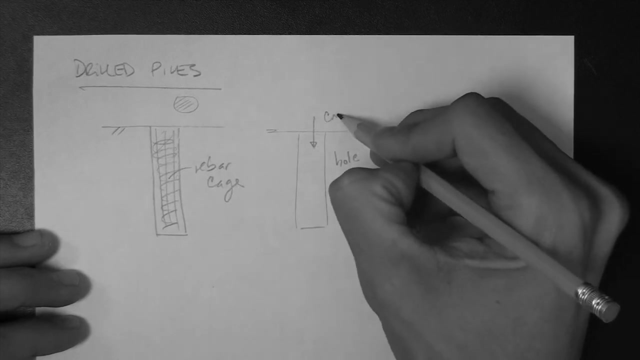 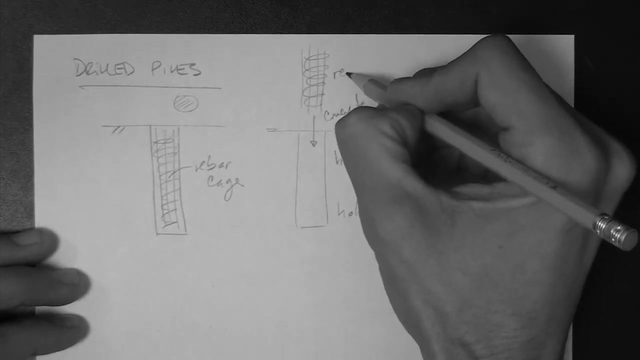 links to videos that show you how this is done, Okay, And show you augers, et cetera. But basically you dig a hole, okay, You fill it with concrete and then you insert a rebar cage- okay, that has been constructed. 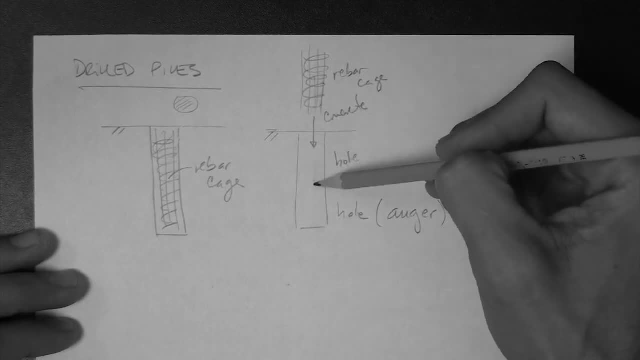 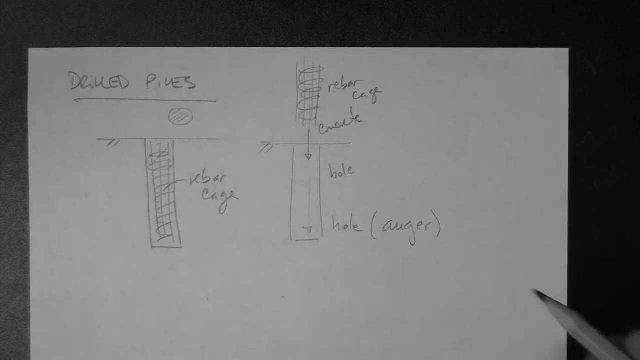 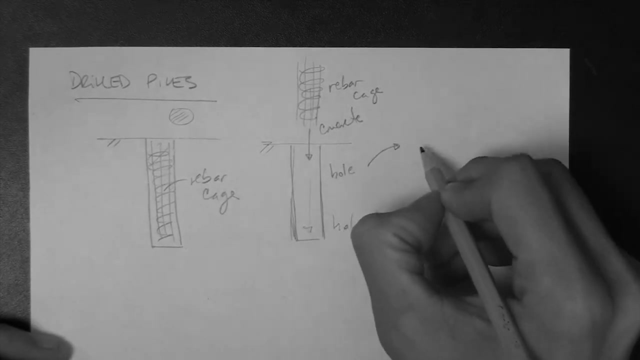 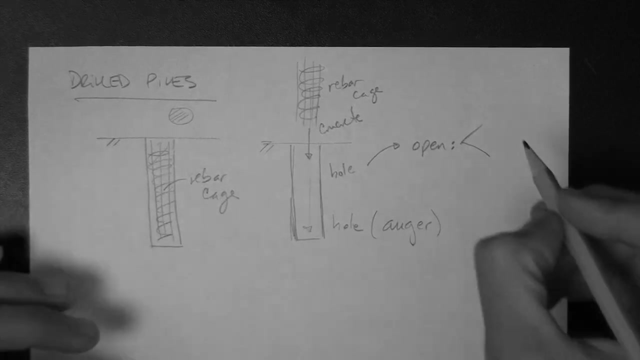 outside: okay, You insert it in, dip it into the concrete- okay. So there are different ways, that again, that this is done. So the major challenges are keeping the hole open, okay. So for that, to keep the hole open, there are essentially two things that are done. 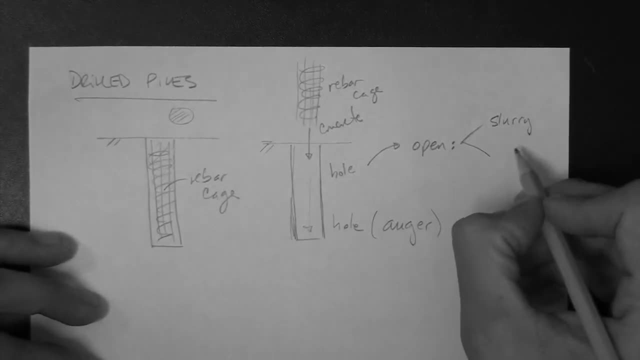 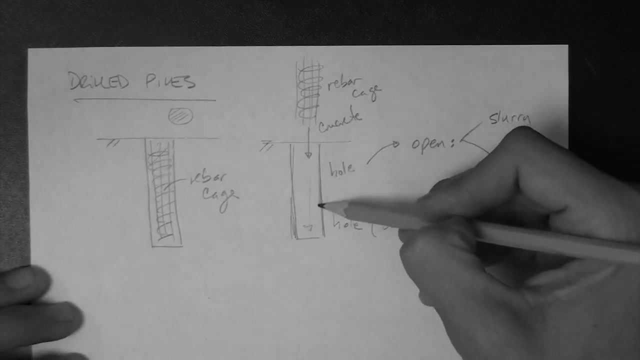 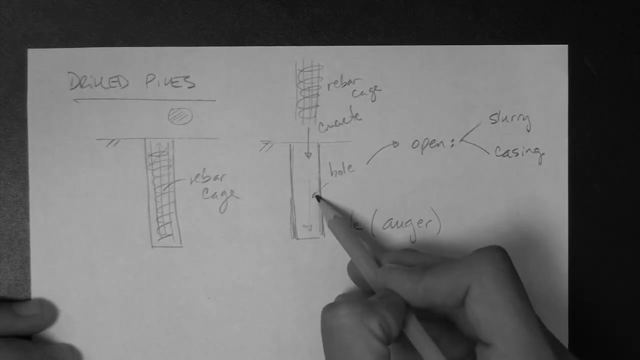 One is to use a slurry and or the other one which is to use a casing. okay, A casing is essentially a steel tube that is pushed in so that it creates the sides of the hole so that the soil doesn't cave in. okay. 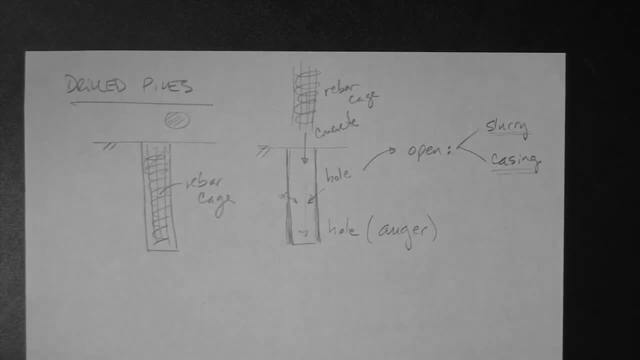 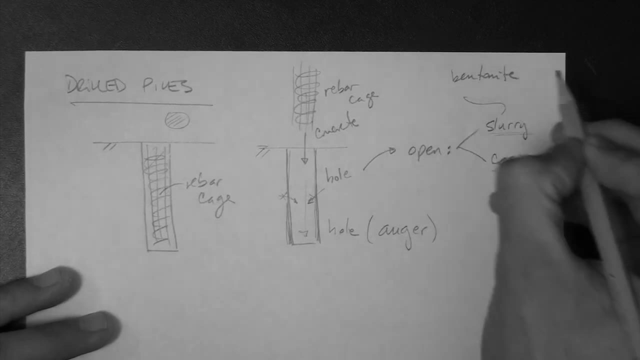 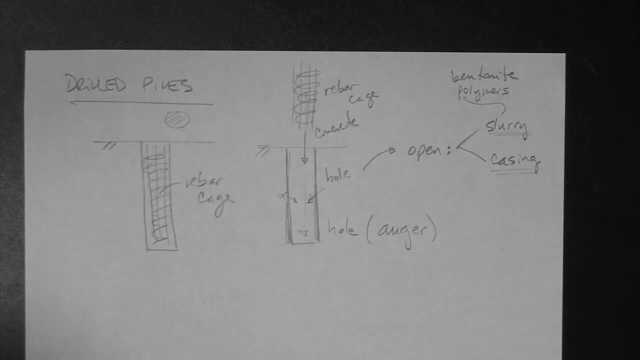 And a slurry is essentially a mixture of different materials. Predominantly, slurries have a clay that is called bentonite, although there are other slurries that are that contain polymers. And what slurries are? a slurry essentially is a mixture of water, polymers and concrete. 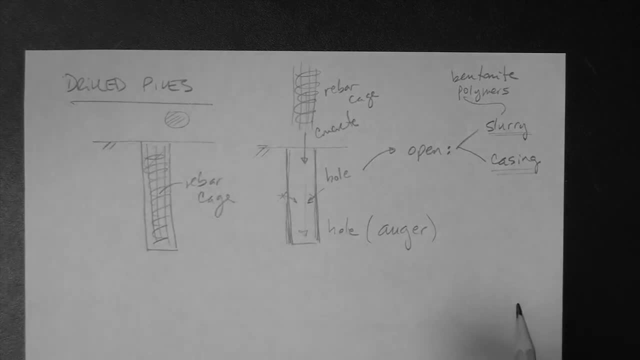 Okay, Sometimes they have polymer, sometimes they even have oil, bentonite, et cetera into a gel, And a gel or a gel-like kind of like a viscous substance or fluid that then is poured into the hole- somehow there are different ways- and it keeps the hole open, okay. 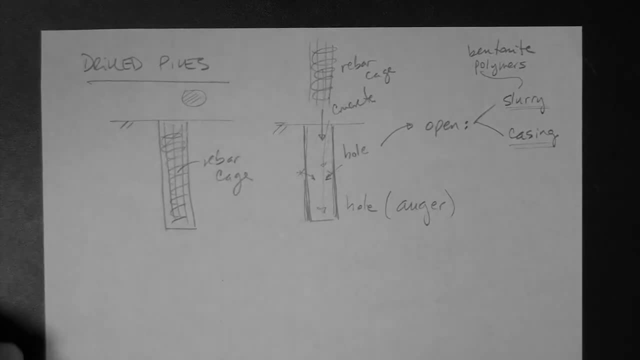 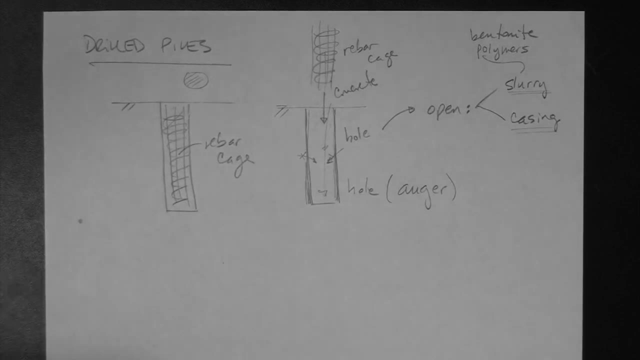 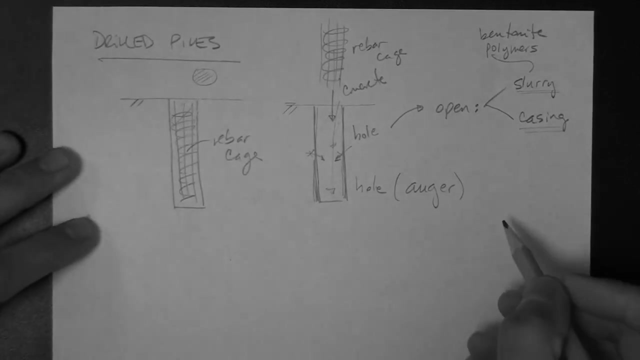 So essentially, that's in a rough sketch. This is a rough sketch of drilled piles. Again, I'm going to provide some examples. Okay, I'm going to provide some links to videos that are going to show you exactly how this is done: time lapses and things by different companies. 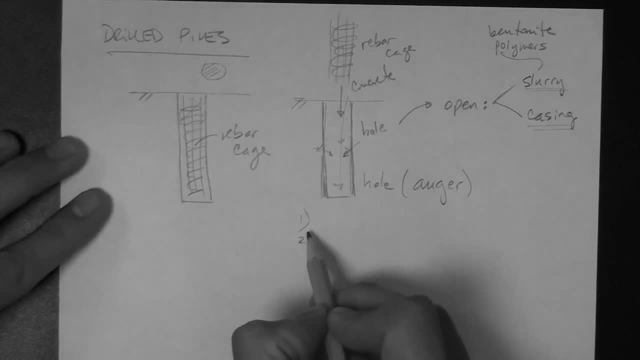 I'll provide that. But just to finish up here, essentially the relative or the advantage of this type of situation or type of pile is that it's silent relative to the hammered or driven pile. okay. Also, very large capacity: Okay, Okay. 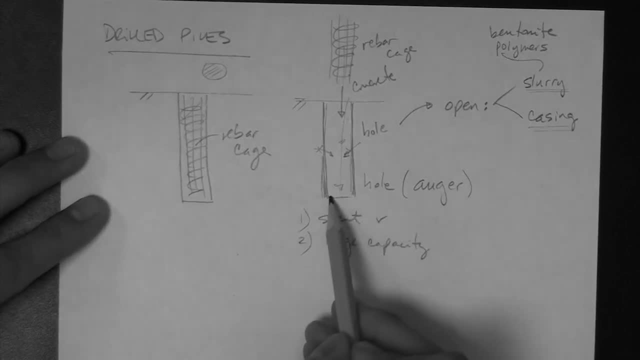 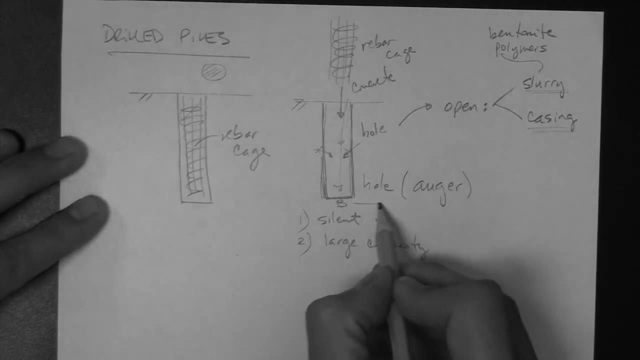 And the reason is that they can be made very, very large. The B can be huge, okay, And I'll provide some videos on that or links to. And then number three is essentially that these are more time consuming, So it's slow construction. let's say: